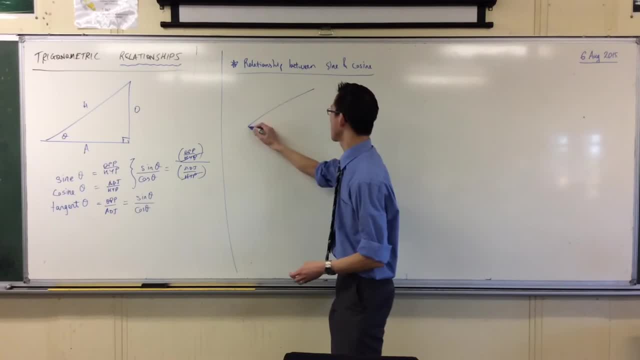 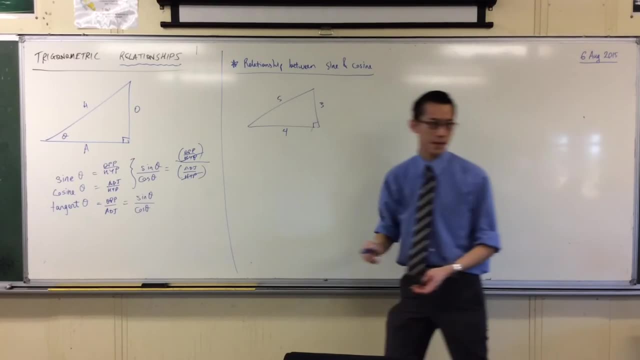 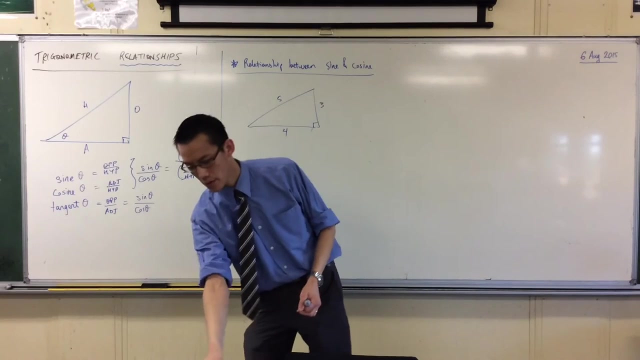 This time let's put in an actual triangle, And I said 3,, 4, 5 before, so let's just draw that guy, because he's pretty easy to draw: 3,, 4, 5.. Now we know enough to work out unknown angles at the moment. So if you haven't already, because we have said we're in trig at the moment, get your calculator out. 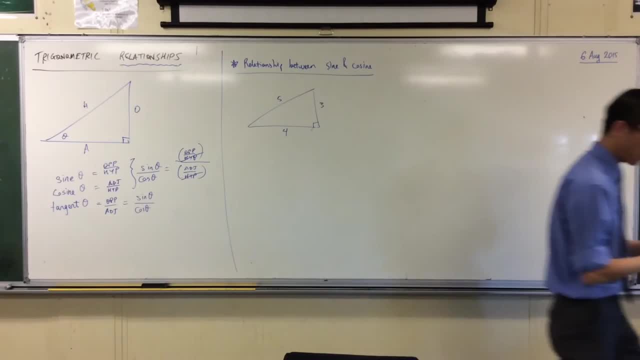 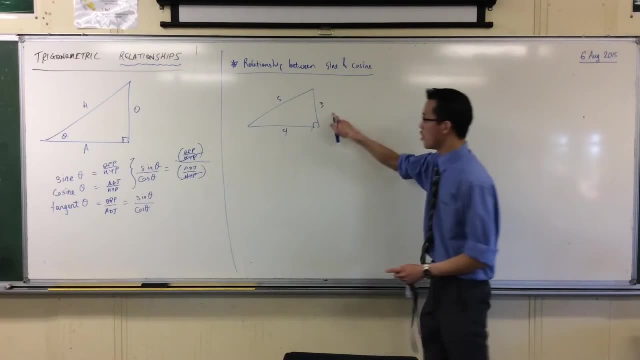 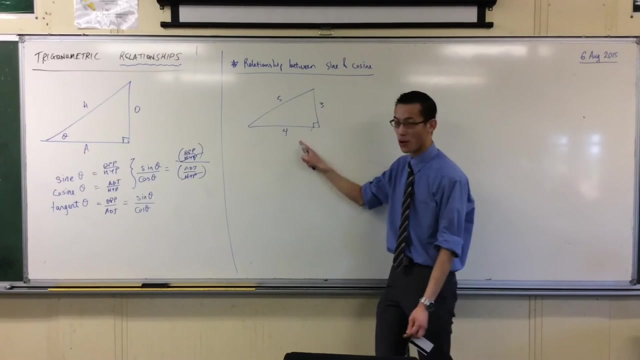 And you see how I marked this bottom left angle as theta before. Now that I know what these sides are, I can actually work out the sides of this angle. There's lots of different ways to do it, because I have all three sides. I can use sine or cosine or tan. I want you to pick any one you like. 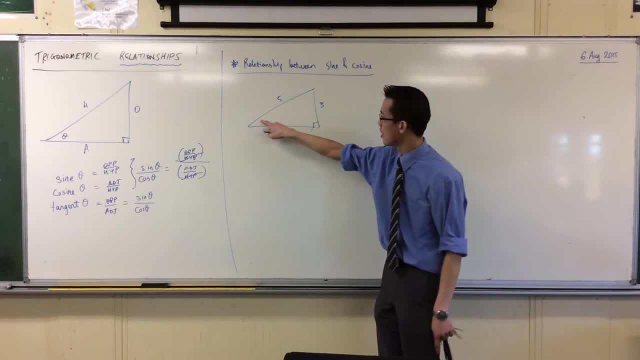 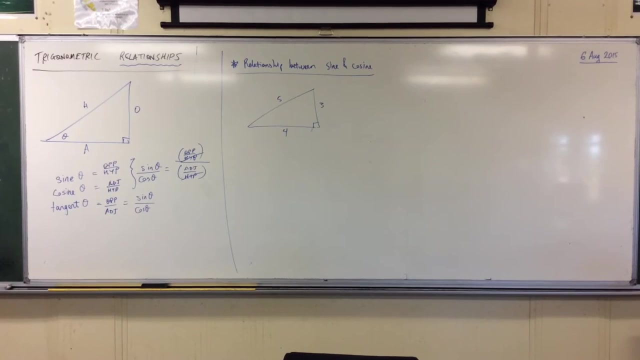 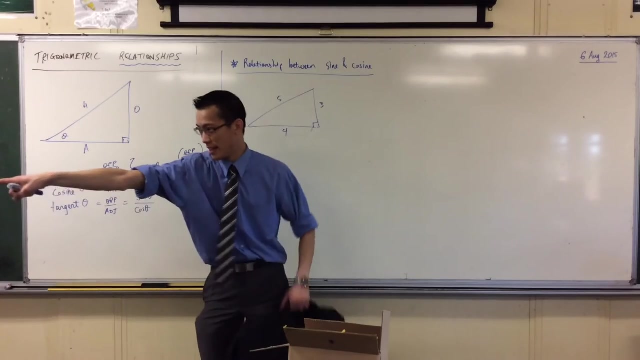 And just tell me what the size of this angle is, or write it on your page to the nearest degree. That'll do Nearest degree, So you don't need a calculator. Good morning mate, Come in. You're going to need that table and this chair. 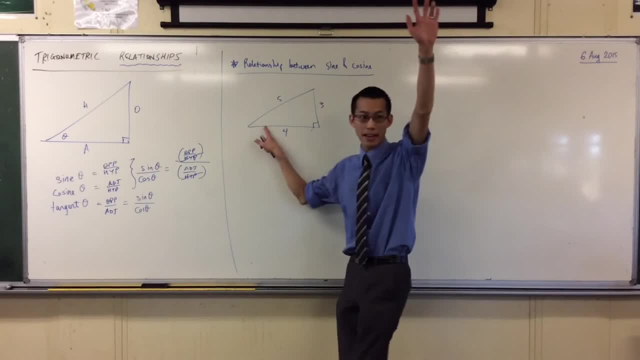 Don't say it yet, but who's got an angle for that? Who's got a size? Yeah, Okay, good, So let's see. It's Ivan. right, Ivan, What angle did you get? nearest degree mate? 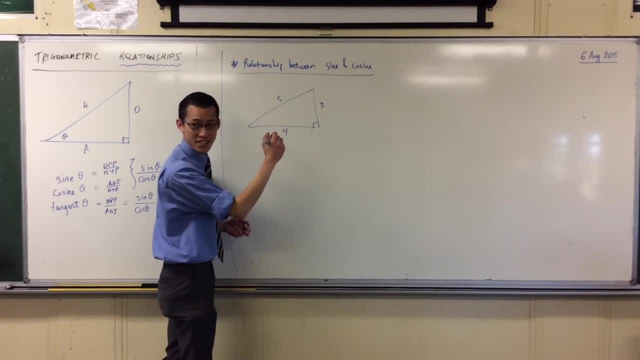 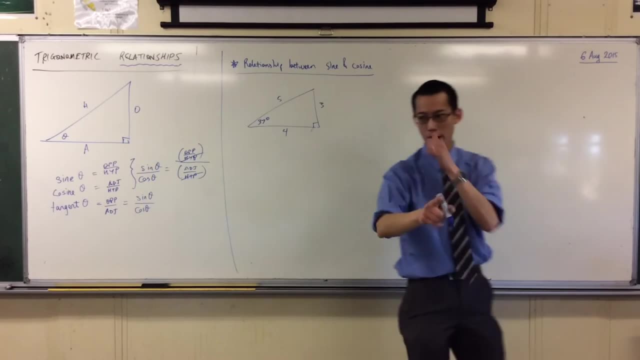 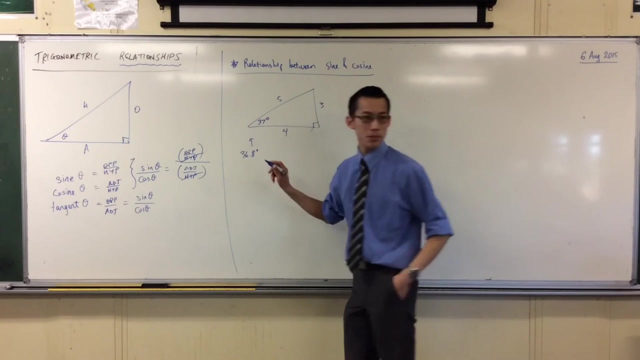 36?? Does that match 37?? Yeah, okay, So we're going to get 37, right, Watch out for that rounding. Why don't we just make a point on that, right? What do you actually get as your decimal 36.8.. So clearly, that's rounding up. Yeah, Okay. 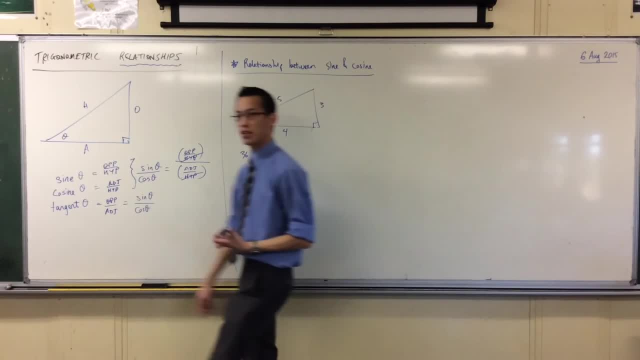 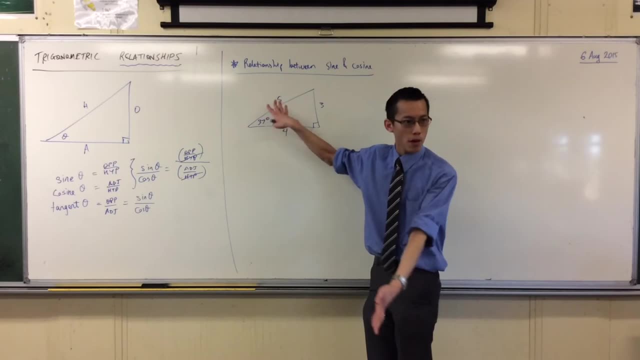 So you have 37 there. It's worth noting. I did mention you can get that 37 a variety of different ways, right? For instance, I could say, if I don't know before I knew what that angle was, we'd just call it theta. 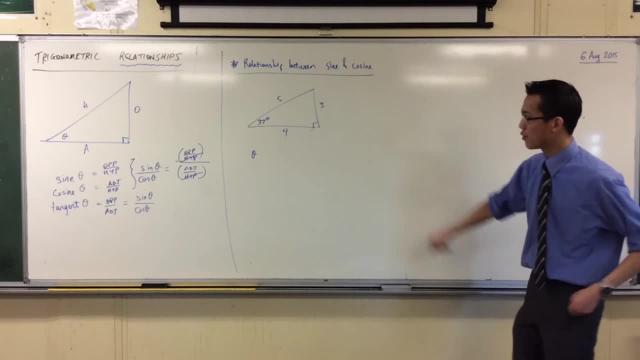 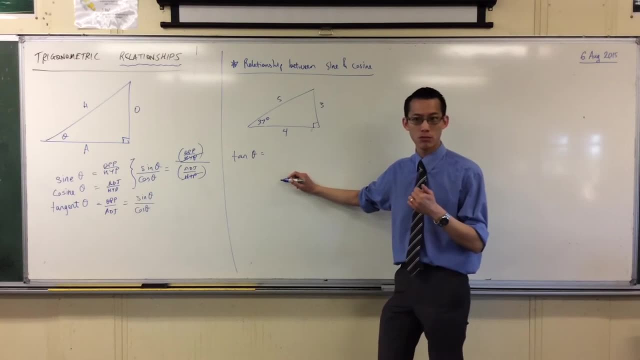 I could say: well, I know, for instance, I know the opposite and adjacent sides right, I know the opposite and adjacent. So I could have said: tan theta is equal to opposite or adjacent, 3 or 4, right. 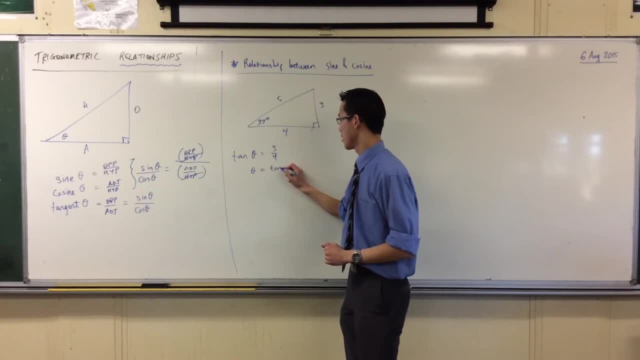 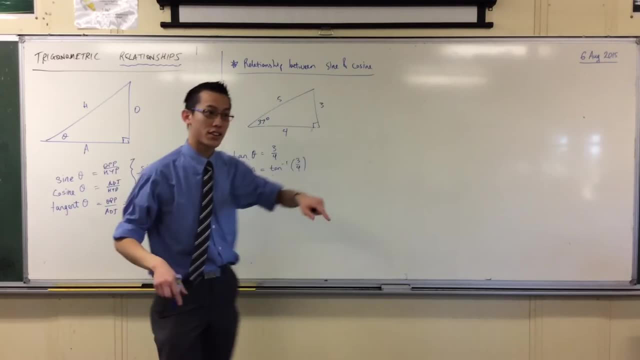 So I could have punched it into my calculator. Theta equals tan with a minus 1.. Does anyone know what the proper name of that is? Tan? yeah, I'll do that. Tan inverse- Very good, Yeah, tan, almost Tan inverse. Tan inverse: It's trying to do the opposite of tan, which is why it gets rid of the tan on this side. 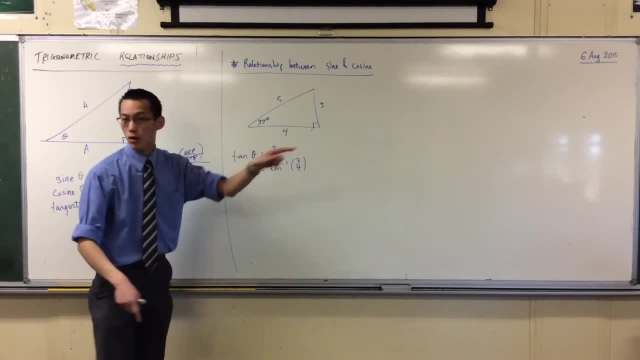 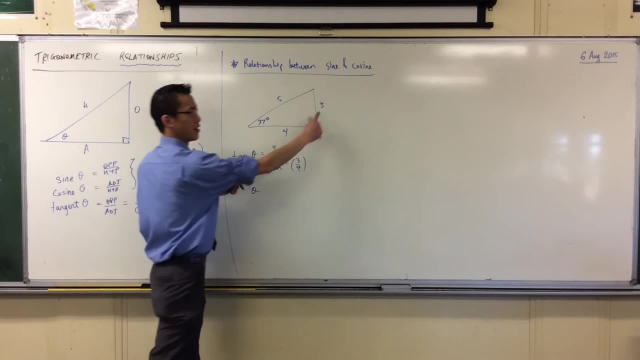 Yeah, And now it would have popped your 37. That's not the only way you could have done it, though, right? If I come back to theta, I can say I know the opposite and hypotenuse. So which ratio is that? 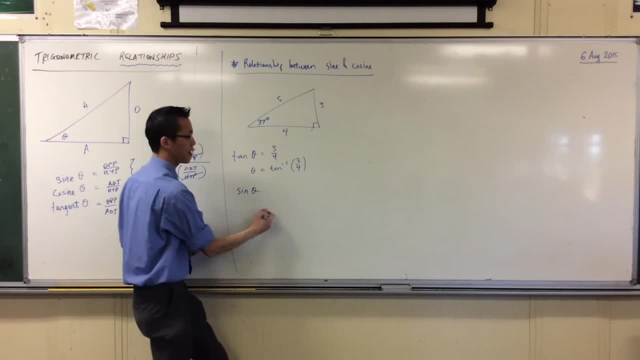 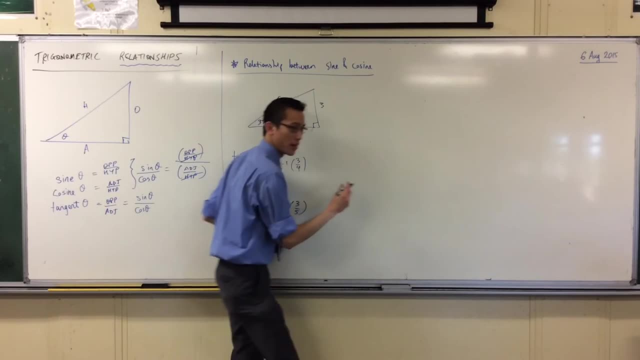 Sine, That's sine. So I could have said sine. theta is 3 fifths, So I could have used sine inverse and I would have gotten the same answer out. Okay, All right, now, that was just an aside. We've got 37 now. okay, This is a wide-angle triangle, so that's 90.. 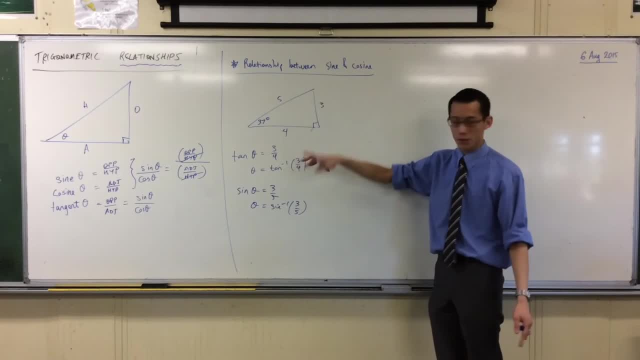 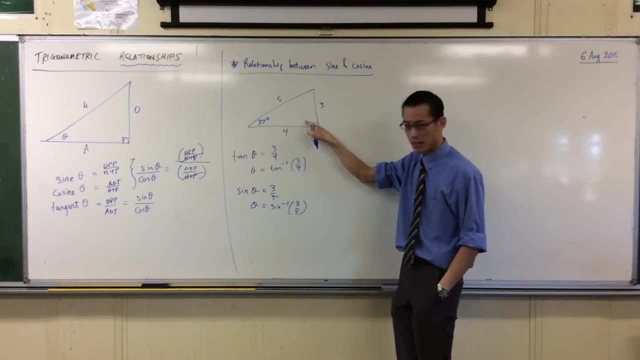 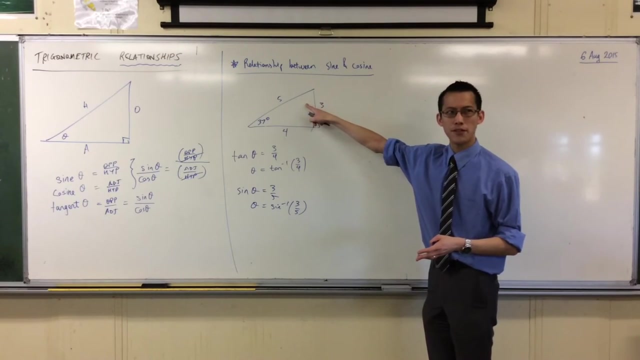 So without using trig anymore, like you've done. enough trig. what's that angle up there? 90 plus 37.. It's going to be well, this plus this plus this should give me 180 degrees, right, Okay? So, if I'm doing my numbers right, that should be 53.. 53? Okay? 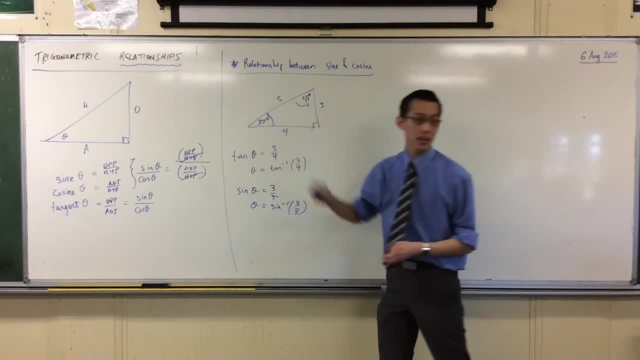 Bless you, Bless. you. Now got a couple angles there, right. Our 37 and 53,. 37 and 53, they're related to each other. Does anyone know what the name is? It starts with a, C, the name that relates those two together, because they add up to 90 degrees. 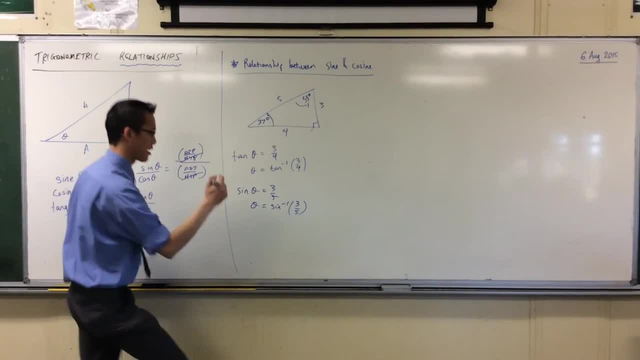 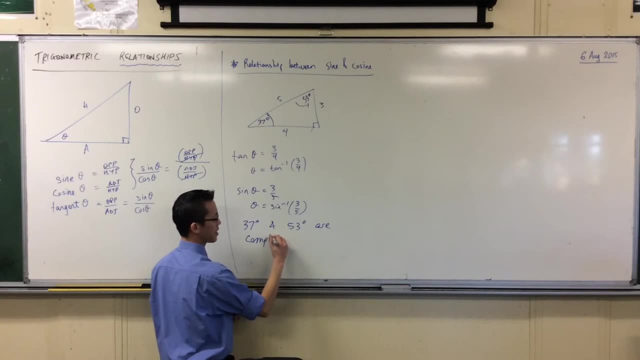 Does anyone know what that's called? They're called complements, okay. So down here I'm going to write 37 degrees and 53 degrees are. you can say it a couple of ways. You can say they are complements, or you can say they're complementary angles. 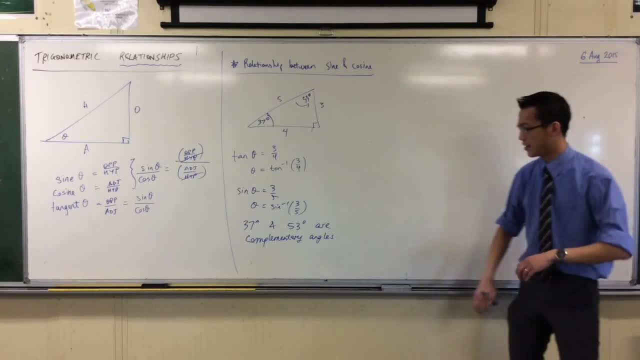 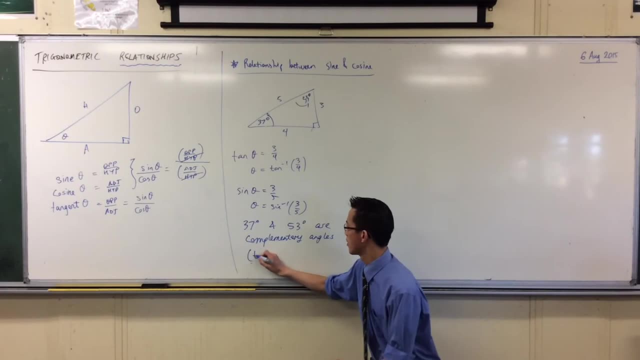 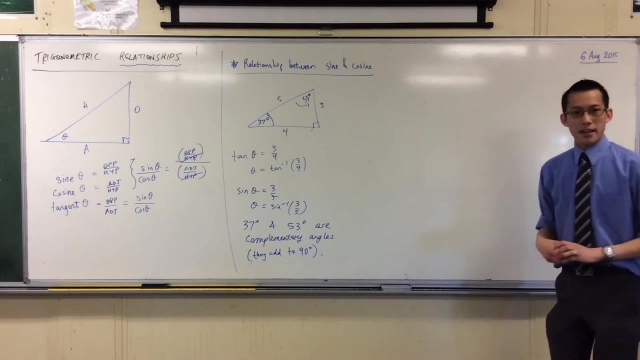 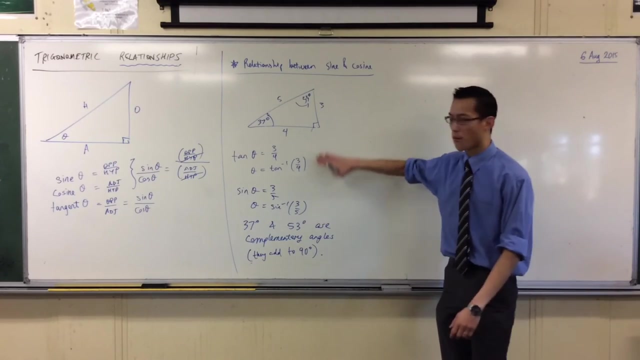 And we mean complementary with an E, not like complement, as in nice haircut, but complement as in. they go together, they match up. Okay, They're complementary angles, which means they add up to 90 degrees. Now remember I said to you: okay, I can look within this triangle, I know all the sides, I know all the angles, so I can say a variety of things about all the different trig ratios in here. 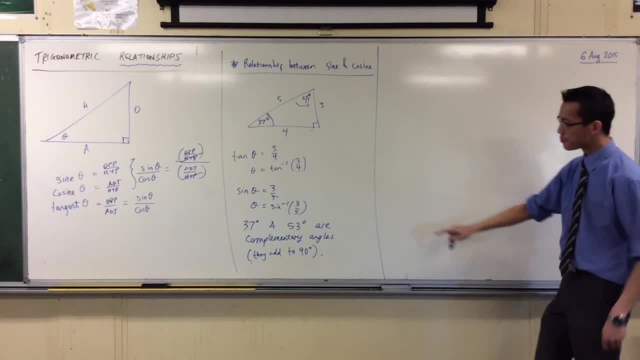 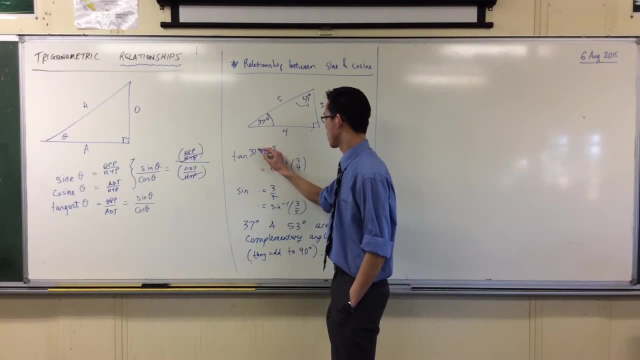 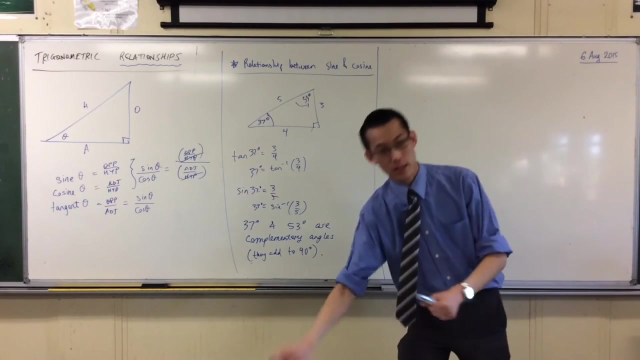 Okay, So I'm still going over here. don't make a new heading. I know what theta is. right, You told me it's 37, yeah, So 37 degrees, 37 degrees and so on. okay, Now here's what I want to focus on: this guy down here sine 37, okay. 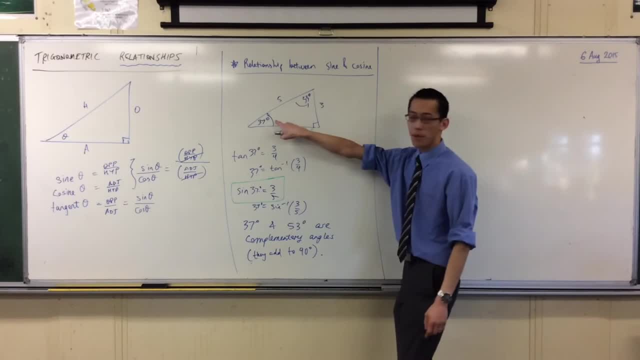 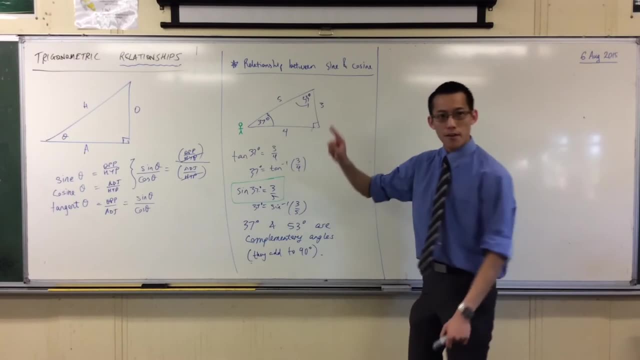 3 over 5,, 3 over 5.. From the point of view of this angle- over here I'm going to put a little man there- right, There's my point of view, my perspective. okay, From his perspective, this is opposite. on hypotenuse, you agree? 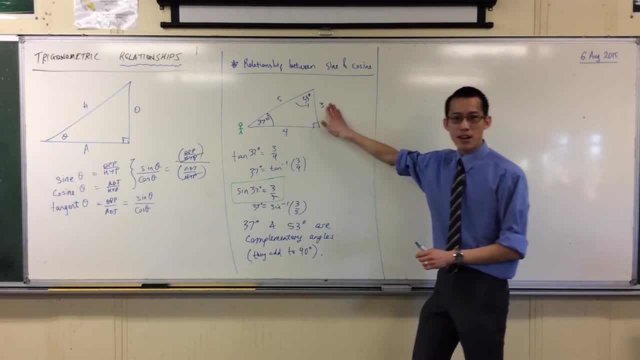 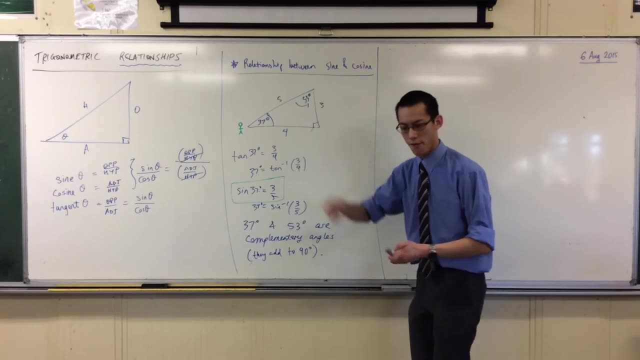 And that's why I used sine. You told me to use sine, But 3 over 5 is another ratio, It's not opposite. on hypotenuse, if I'm standing somewhere else, If, for instance, different color, I stand over here, 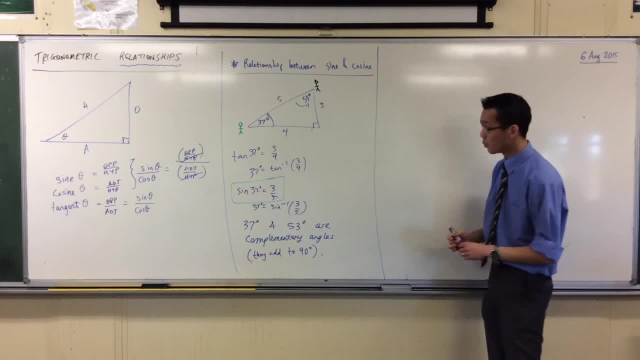 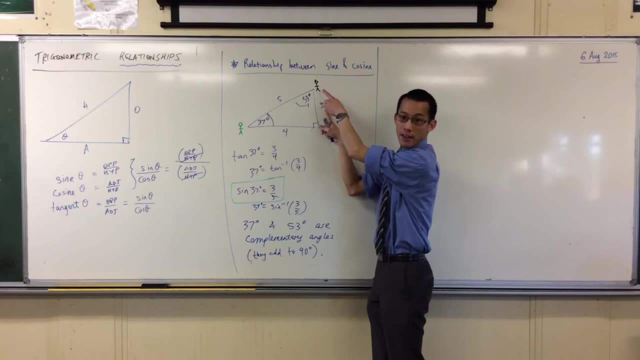 3 over 5 is no longer opposite on hypotenuse, is it? From that point of view, what is it Adjacent? Yeah, this 3 is adjacent. It's neighboring that angle up there, the man that I've drawn in black. 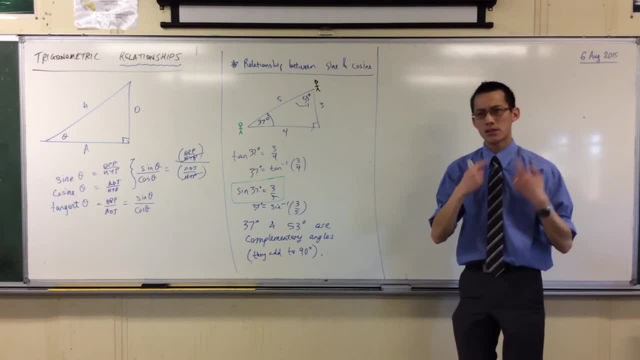 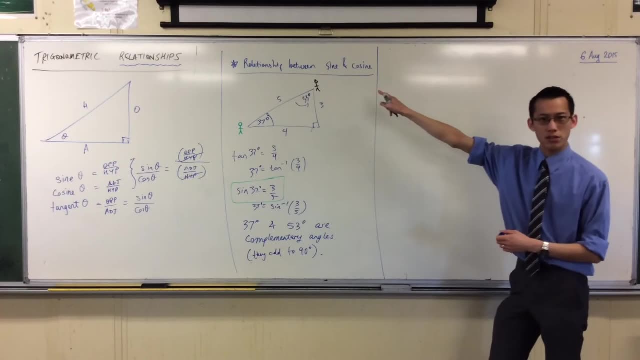 3 over 5 is adjacent on hypotenuse, So therefore I should be cosine, right? So what statement could I write that matches what you just told me? You said cos different point of view, so it's going to be a different angle, right? 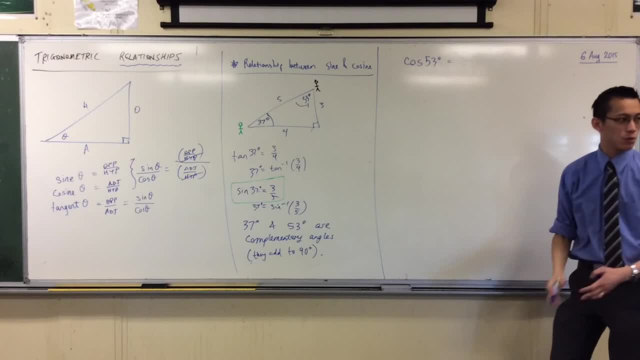 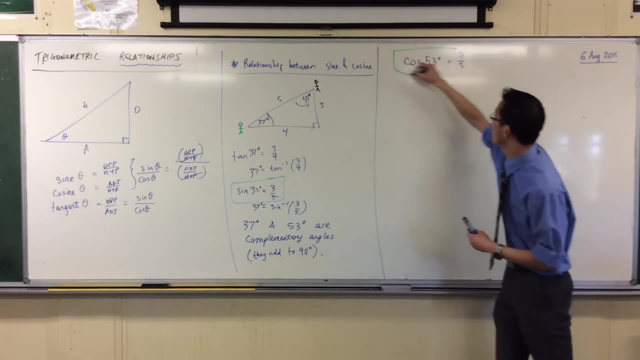 53 is equal to that same 3 over 5.. It's the same thing, okay, So I'm going to put this in green. If you've got colors, by the way, this is enormously helpful so you can see the parallels. 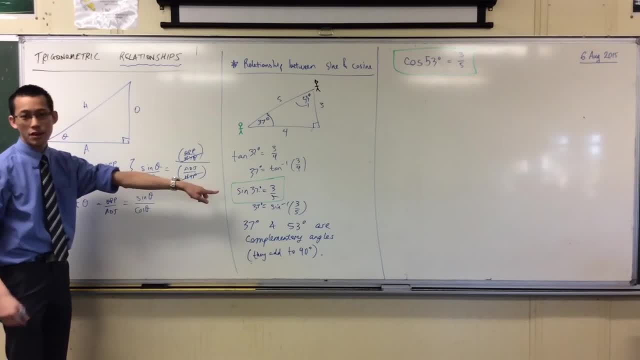 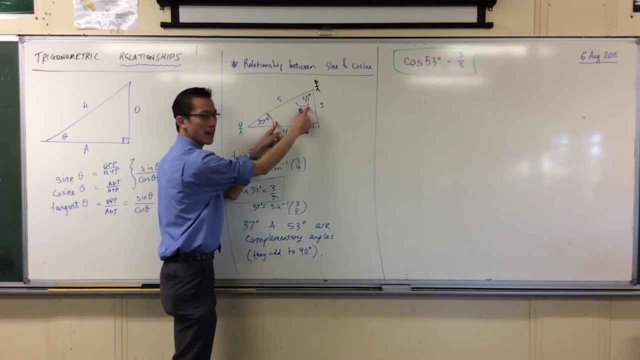 These two things are the same: Sine 37.. Sine 37 and cos 53,. okay, Now, this is not an accident and it's not just a coincidence because of this particular triangle that I made These two angles. tell me again, how did you work out this angle from this angle? 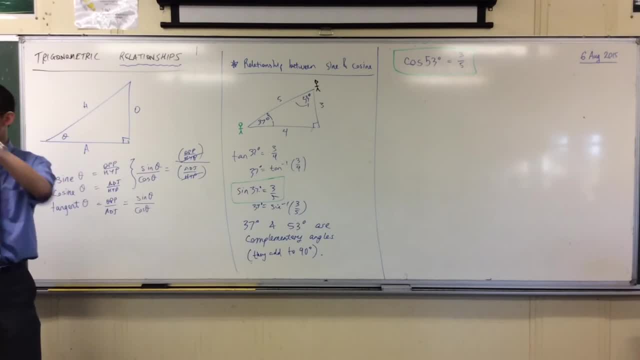 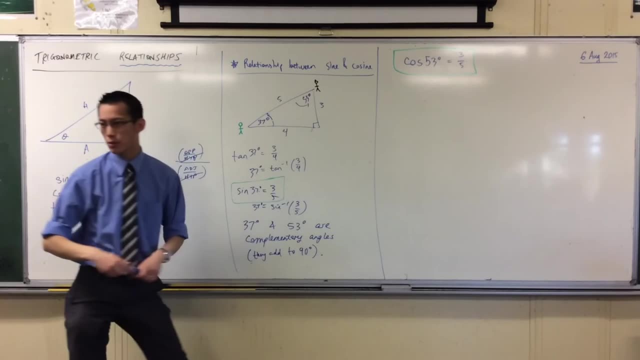 What property did we use? We used the angle sum of a triangle. right Now, every triangle shares that property, Every triangle, they all add up to 180 degrees. So if I had a triangle, if I had a triangle that was maybe a bit smaller, 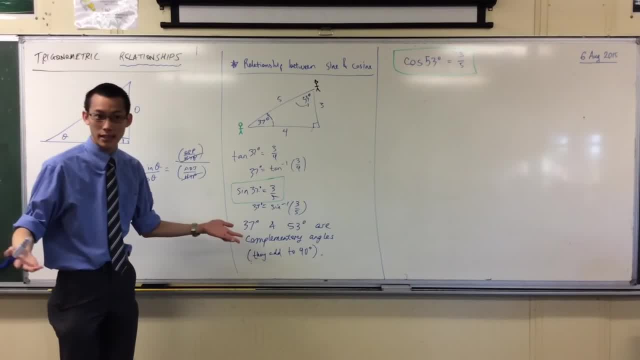 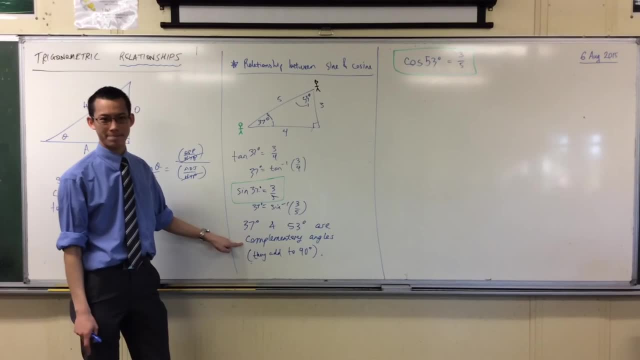 maybe had a smaller angle over here, like 36 or 30 or 18, right, That angle up there is going to change, but it's still going to be complementary to whatever's here in the corner. You see, they're always going to add to 90?. 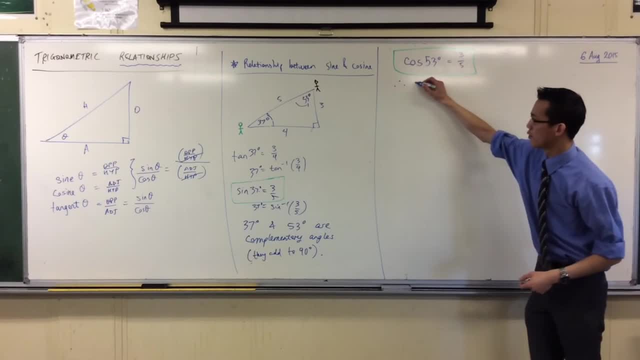 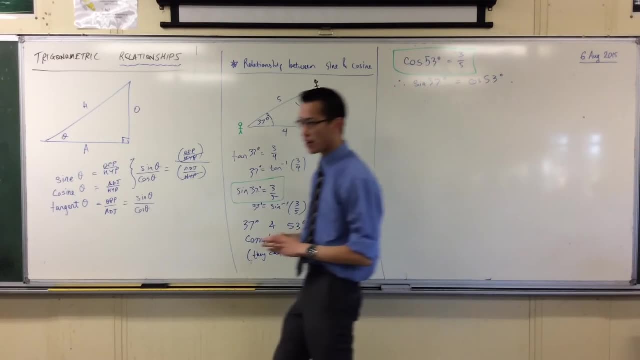 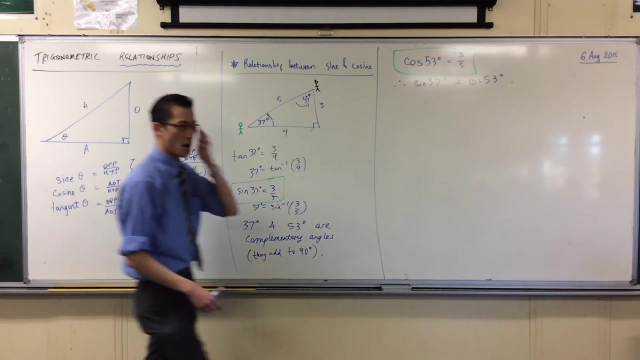 So the fact that these two are identical, right? Therefore, sine 37 equals cos 53.. This is not a coincidence, right? In mathematics, we're always looking for patterns, right? This is actually always going to be true, provided that these two angles are complementary, right? 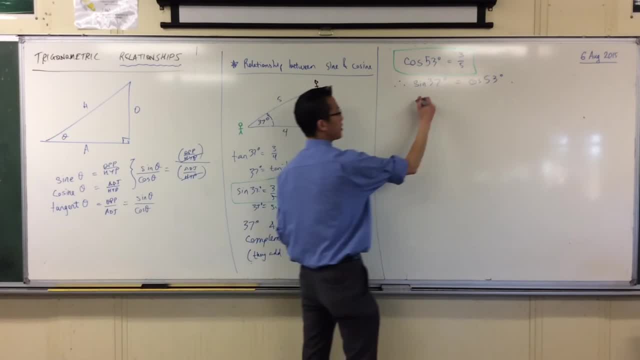 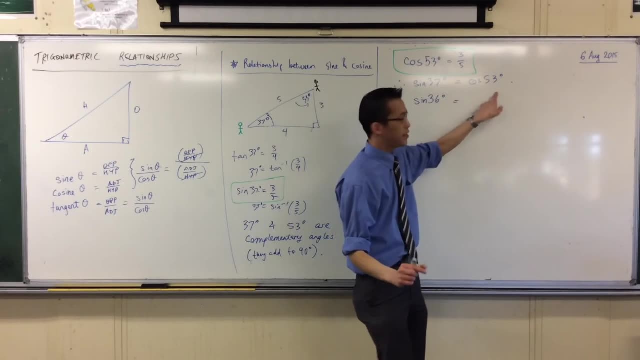 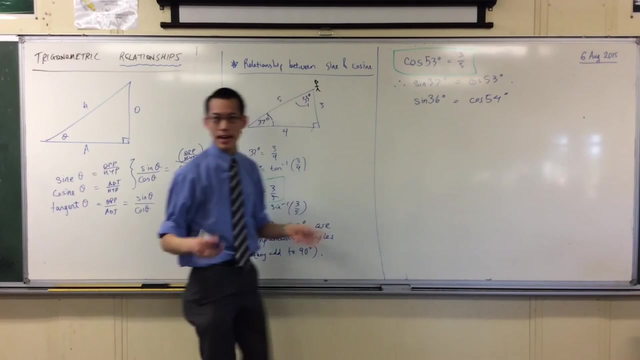 So, without drawing a new triangle, I could say sine 36. If I make this angle a teeny bit smaller, then this angle will be a teeny bit bigger, right? They sort of have to match up together. They must add up to 90 degrees. 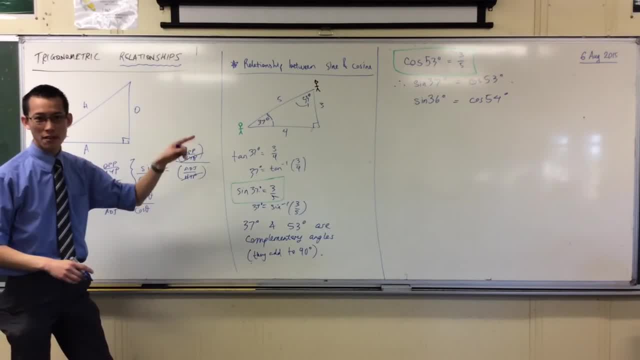 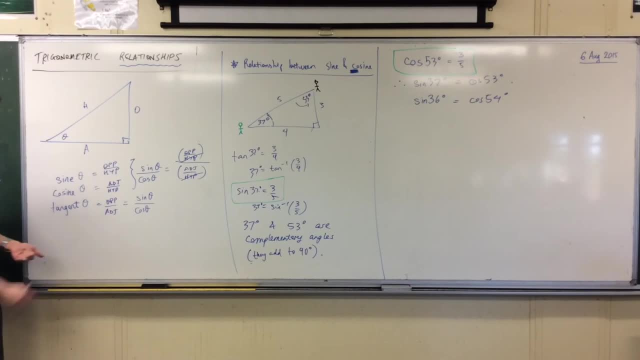 They must be complementary. Okay, They must be complementary, and that's what the cos stands for in cosine. Cosine literally means it's the complement, complement, this complement of sine. Okay, Let's generalize this. This is just for, like, two angles, right? 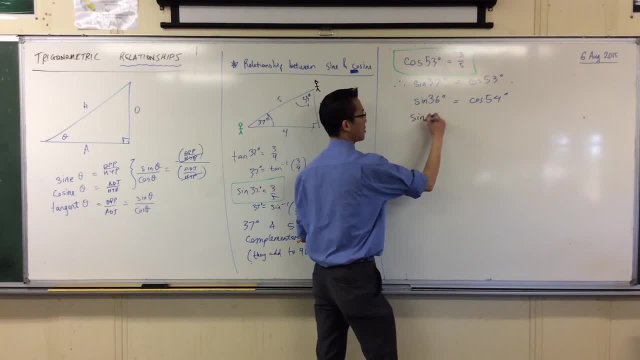 But I can say this for any angle. I can say: sine of theta, whatever theta you like, okay is going to be equal to now. if I don't know what theta is, how am I going to say what the complement of theta is? 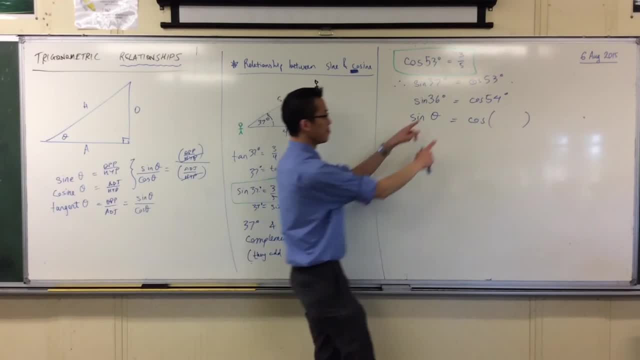 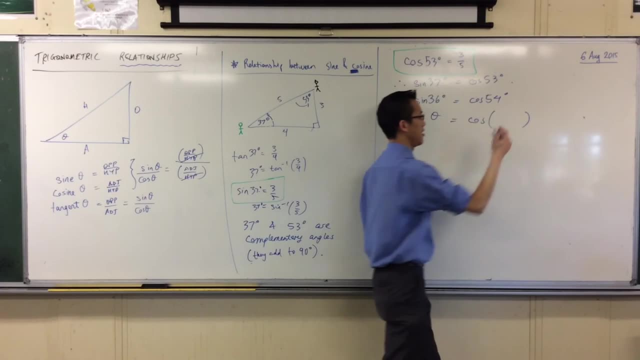 if I don't know what its value is. Yeah, very good. The way I get 54 is it's 90, take away 36.. The way I got this was 90, take away this. right. So I'll say 90, take away that, okay. 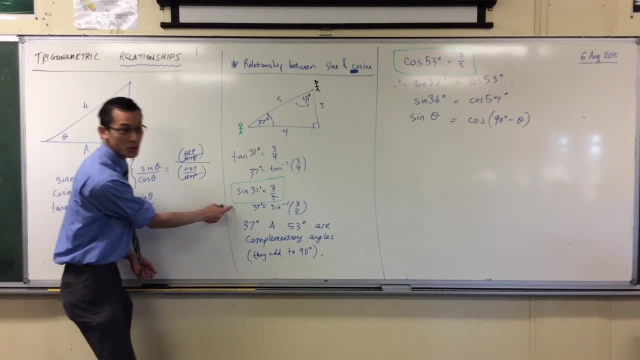 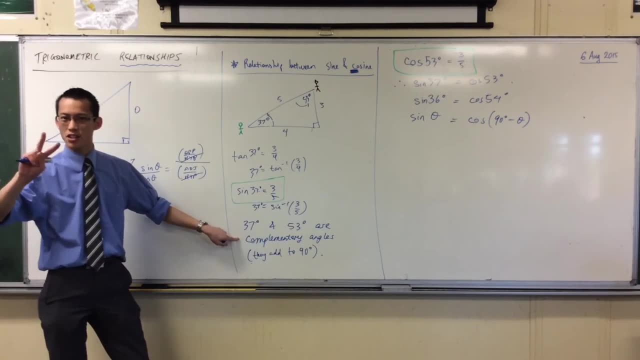 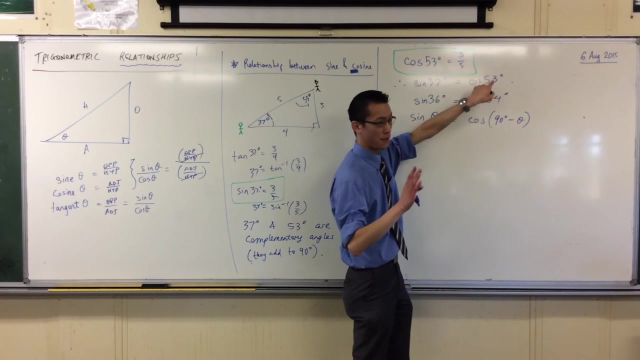 Now it doesn't take too much to see. For instance, I started with sine and then I noticed it about cosine. But I could have done it in reverse. right. Complements are a symmetrical relationship. right? So to say 37 is the complement of 53 is exactly the same as saying the complement of 53 is 37.. 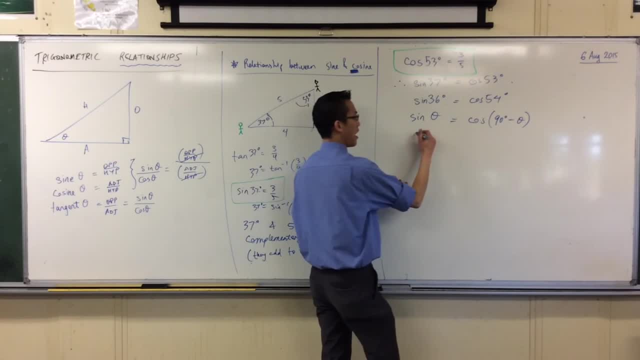 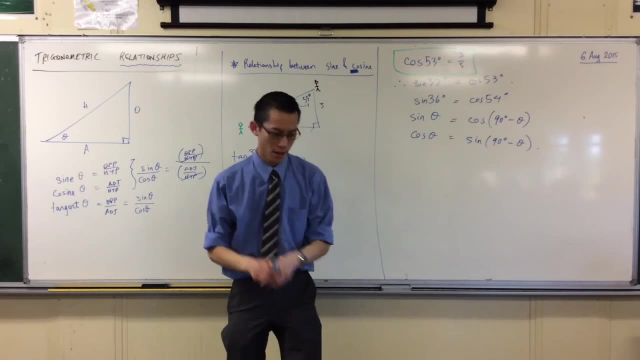 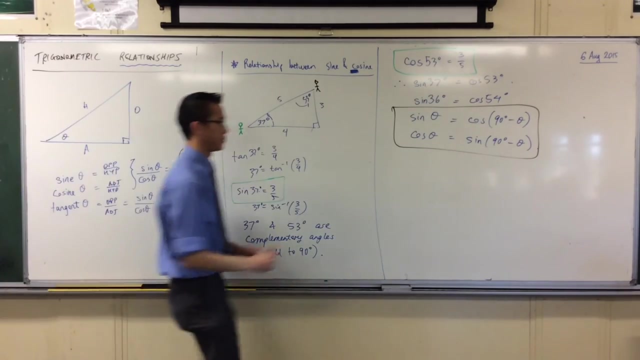 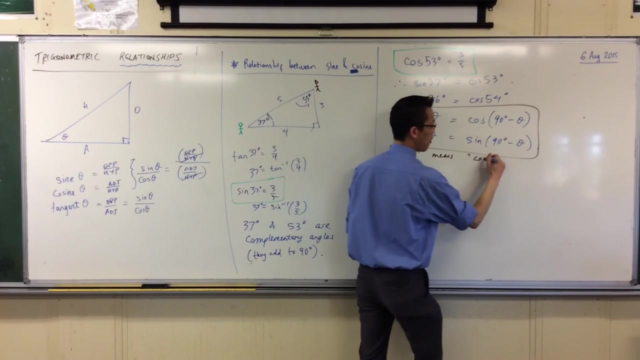 So I can say this the other way around as well. I can say: cos theta will be sine of 90 minus theta. Okay, Put a big box around it, because this, this is the relationship between sine and cosine. Cosine means it's short for the complement of sine. 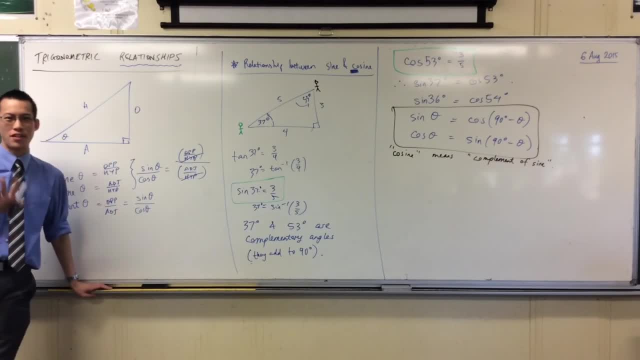 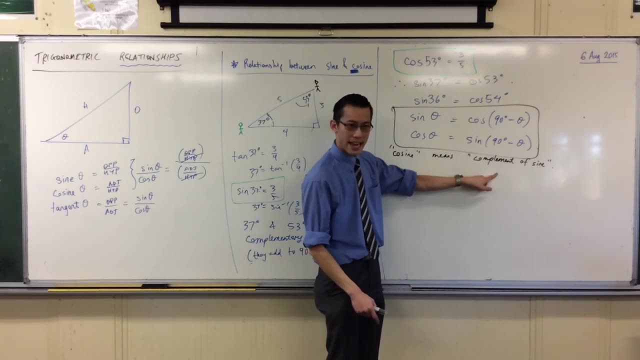 Whenever you discover the name of something, you've always got to push on that a little bit. You don't have to necessarily understand why something is named what it is, but more often than not something's name will reveal to you something fundamental about what something is. 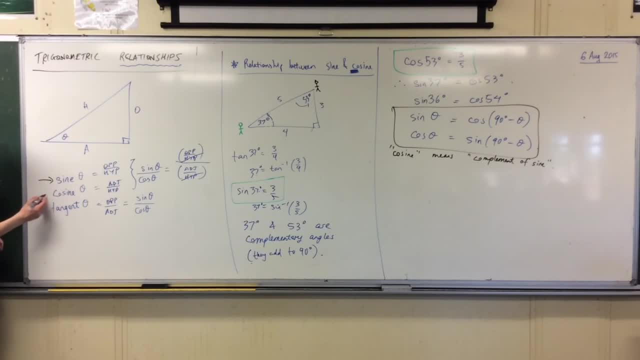 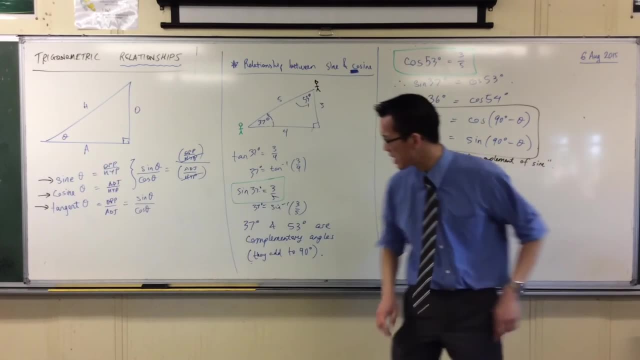 Wow, I think I make that point. We've done one ratio, two ratios. there's a third ratio. You've met this word before, haven't you? What's a tangent, Haven't you? If you, you've got a year seven student. they've never seen this word before, right? 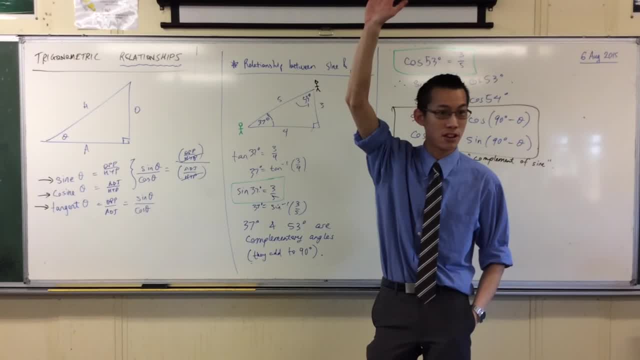 Hands up if you don't have to say it. Hands up if you know what this word means. You got an idea. Okay, let me draw it for you. Yes, circle is exactly right. So you got a circle, okay. 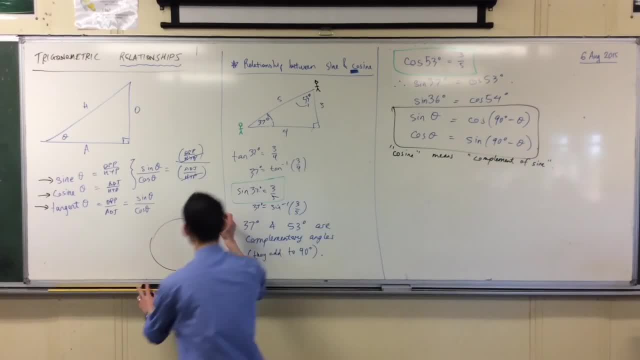 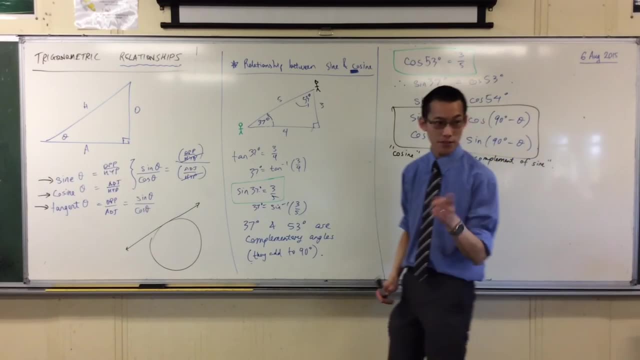 And there's, there's a straight line I can draw That just touches the circle. just touches, okay, Which, in fact, by the way, is where the word tangent comes from. There's another word in our language that we use when things touch, that starts the same way. 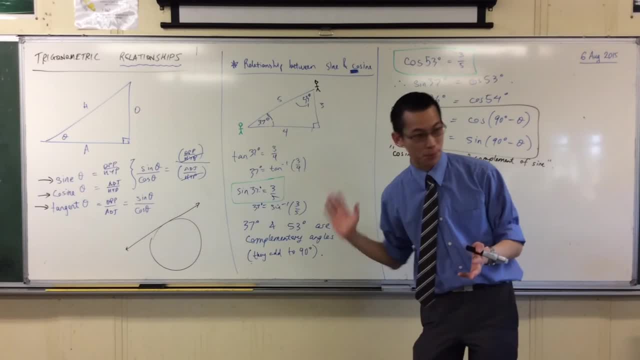 Does anyone know, When you say something is you know it's, you can't put your hand through it like air? okay, A table, we say it's. we say it's tangible, right, You can touch it okay. 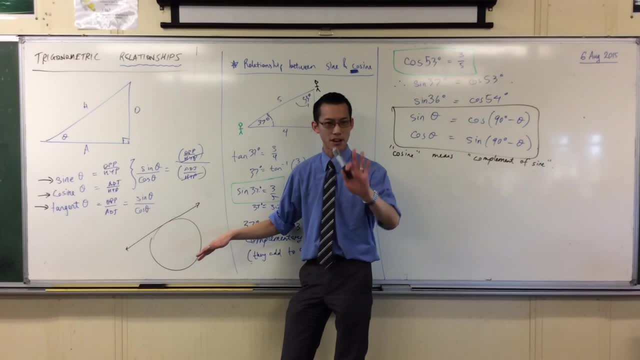 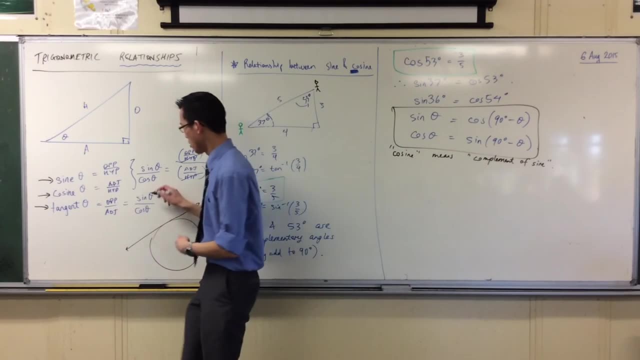 A tangent is just touching a circle And just an open thought for you. and we'll, we'll, I'll give you the answer next time, I promise This is a tangent, This is a tangent. What on earth does this have to do with this? 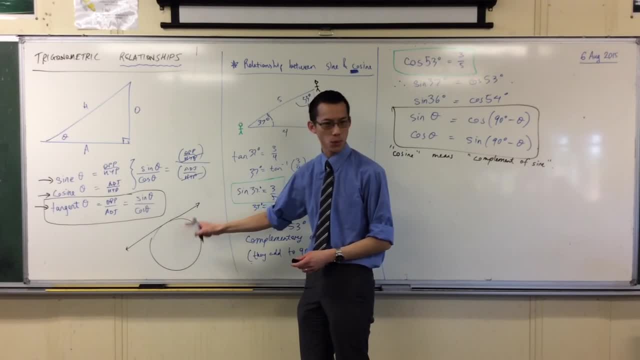 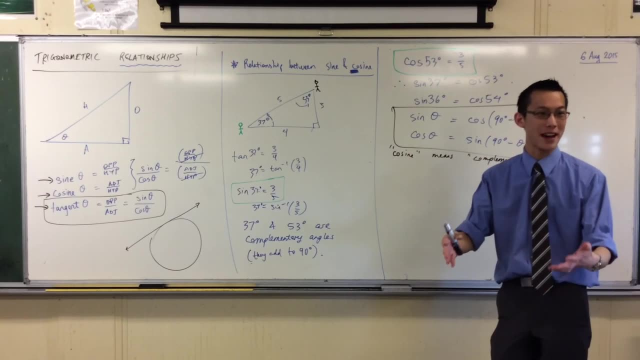 I don't see any triangles in this diagram. What's up with that? Okay, Mathematicians, as you can see, have no problem making up new words for things if we have a new idea, right. But they chose to recycle this old word when they were talking about something in triangles.